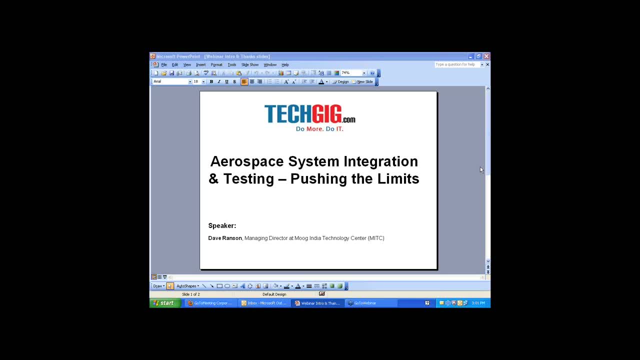 as well as achieving AS9100 certification. Current projects include embedded flight control software and electronics, flight control actuation components and qualification testing for the Boeing 787 and Airbus A350.. MOOC's India Technology Centre is now a centre of innovation for key technologies. 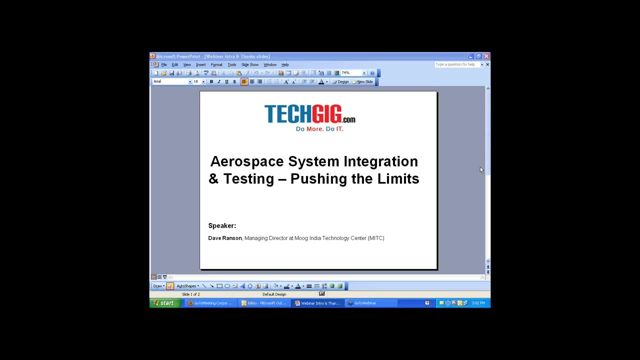 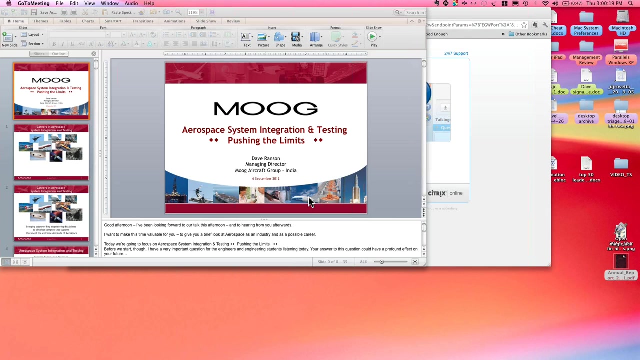 that support aerospace, automotive and industrial controls. So, without further delay, I introduce you all to our guest speaker. Over to you, Mr Nansen. I'd like to make this time valuable for each of you. I'm looking forward to sharing a little bit about the aerospace industry. 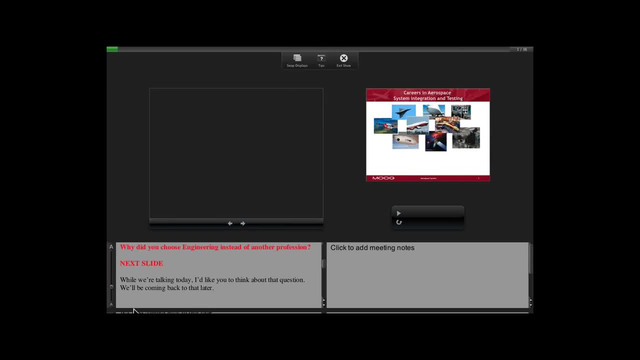 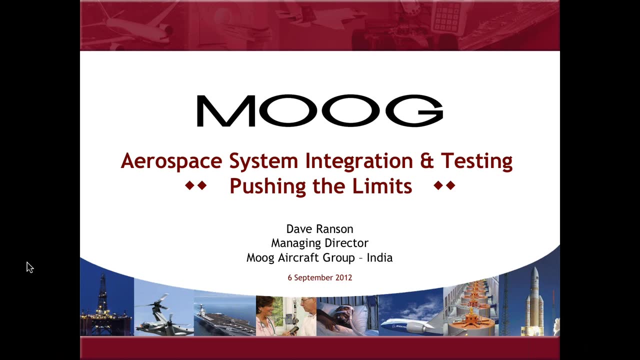 and also about possible careers in aerospace. Today, we're going to focus on aerospace systems and integration, and the testing, pushing the limits. Before we start, though, I have a very important question for the engineers and the engineering students listening today. Your answer to that question could have a profound effect on your future. 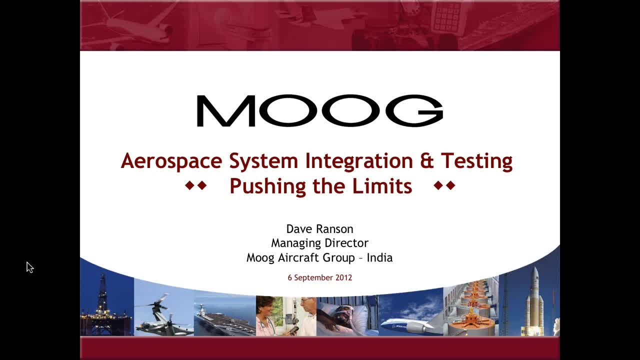 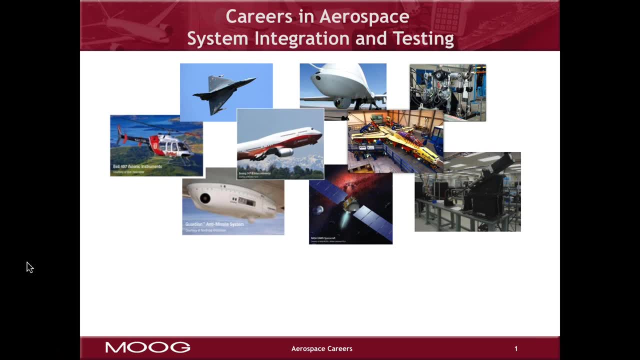 Why did you choose engineering instead of another profession? I'd like you to think about that. while we're talking Careers in aerospace to get us started, I'd like to give you some context for our discussion. During my 30 years of aerospace experience, I've been involved 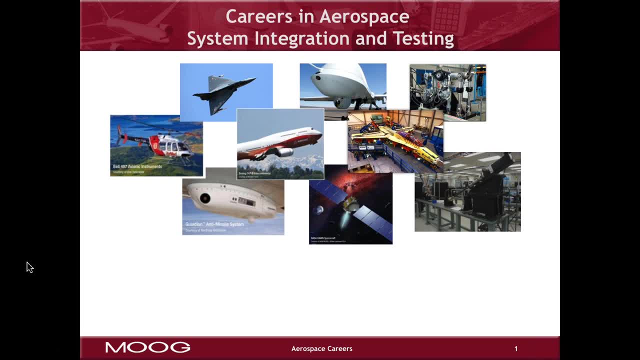 with four different aerospace companies and I've enjoyed being with each of them. I'd like to share some of the things I've learned as we talk today. Also, I'd like to share some of the things I've learned as we talk today. 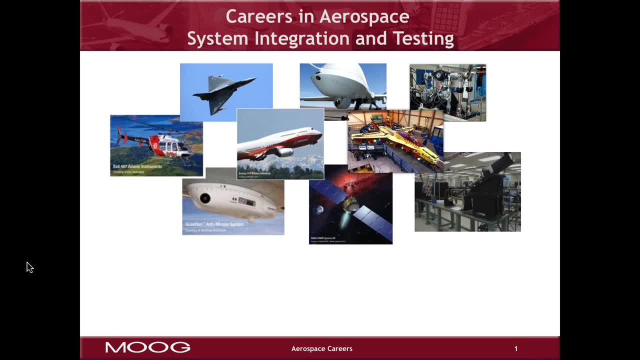 I'd like to talk just briefly about Moog, the company I'm with today, to give you some understanding of the company. It's about 11,000 employees worldwide in 28 countries, $2.3 billion in sales US last year and probably over $2.4 billion this year. 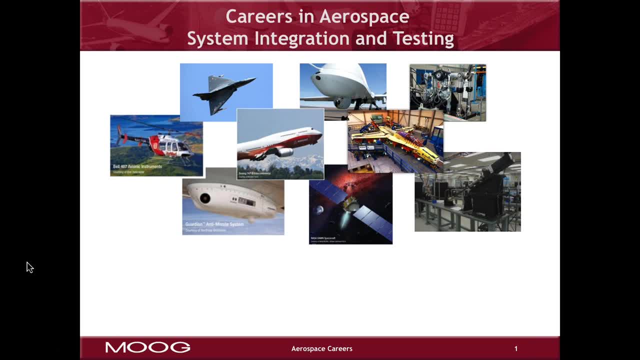 Moog is a worldwide designer, manufacturer and integrator of precision motion controls, And that involves innovation, innovation and innovation. It involves innovative technology solutions that show up everywhere. As you can see in this slide, there are applications of Moog solutions.